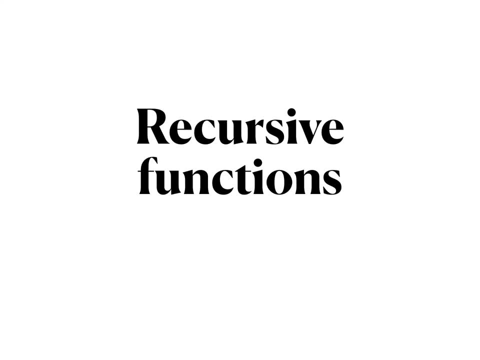 In the previous lecture we saw that primitive recursion is not able to capture all functions that we would deem effectively computable, And one such example was the Ackermann function. So we need to look for ways to expand the class of primitive recursion to capture those. 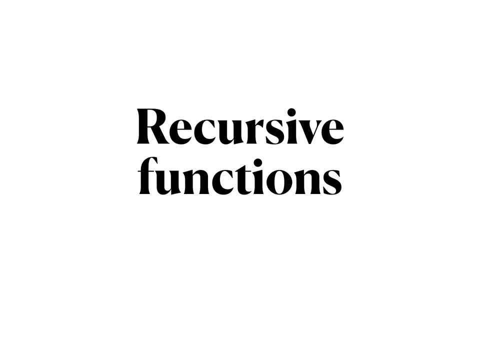 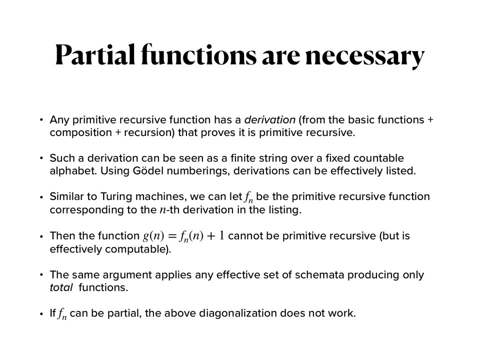 functions, And in this lecture, we will look at one way to expand those, And this will lead to the recursive, or mu recursive functions. Before we do that, however, I want to go over an argument that shows that it is not possible to stick with just total functions, So with 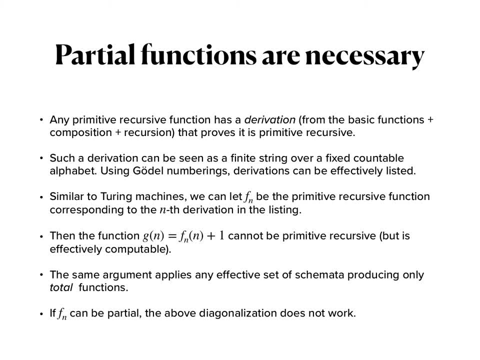 a framework in which every function is defined for all natural numbers if we want to have a framework that captures all computable functions. The reason is that any primitive recursive function has a derivation right. So, as kind of a proof that shows how we can derive this function from the basic functions and applications. 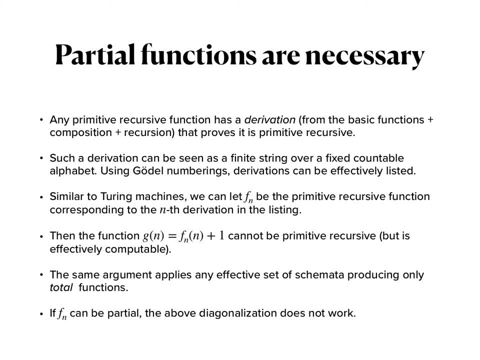 of composition and recursion. Now, just like we did it, we can do it for proofs, We can watch or see derivation, such a derivation as a finite string over a fixed countable alphabet, And then we can apply the whole machinery of Gödel numberings to it, similar to what we did to Turing machines, And therefore, 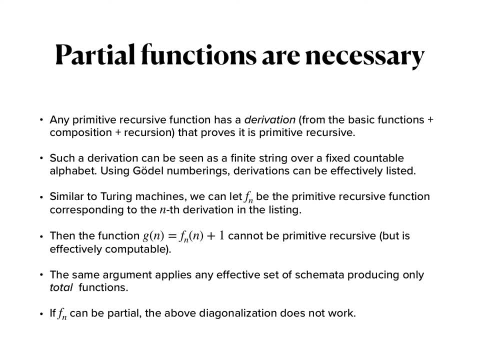 we can effectively number or list all derivations of primitive recursive functions. So we obtain, in other words, a Gödel numbering of the set of primitive recursive functions, And then we can let f, sub n, be the primitive recursive function corresponding to the n-th derivation in the 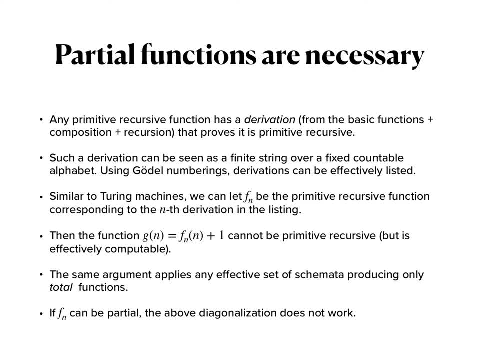 listing. Now we can form the following function: g of n is f sub n of n plus 1.. So this function would be effectively computable because we could just look, produce the n-th function in our listing And compute this function. 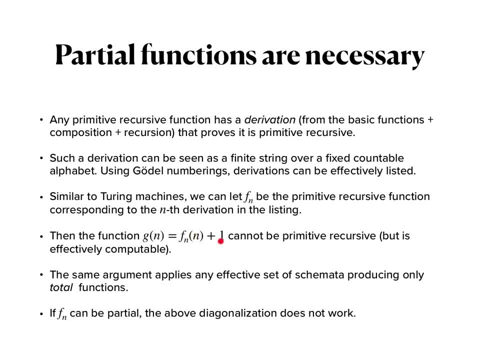 And then we can add a function on input n and just add 1 to it. So intuitively this is an effectively computable function, but it cannot be primitive recursive because we just defined by this diagonalization g to be different from any primitive recursive. 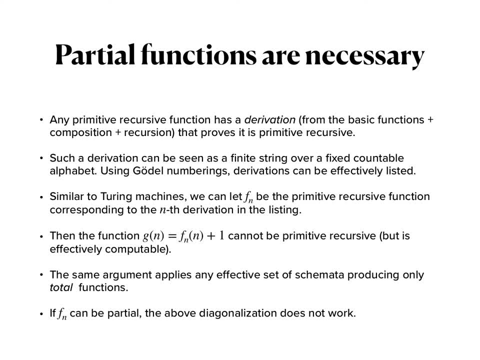 function And there's actually nothing special about primitive recursion here. This argument applies to any schema that we can use to define f sub n. Now we can add a function on input n for any function. I think we can do that. byortic is because there's not a special function, but it's 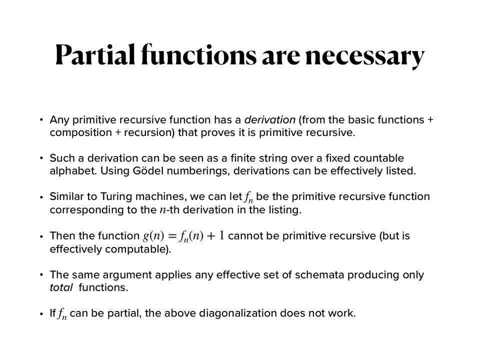 the only one that produces computable functions, The only function that produces computable functions, that produces only total functions, right, As long as we can list them effectively and retrieve a function given on the index in the list, we can implement this function here. 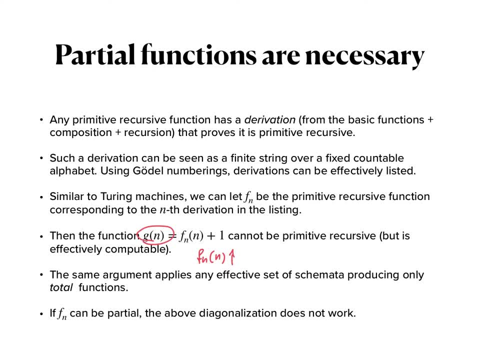 Right. However, if f n can be partial, that means it's not necessarily defined. So if f n of n can be undefined right, Then g n would be undefined Right. Right, find two, and therefore we don't have the diagonalization happening at this point. 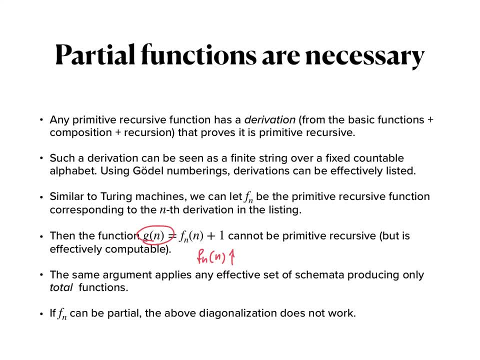 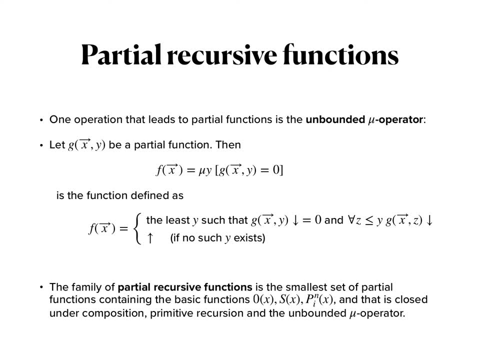 So for partial functions this argument does not work. One operation that can lead us out of the total function and lead to partial function and yet is effective is the unbounded mu operator. We've already seen the bounded mu operator, where we essentially just looked for the smallest witness to a statement. 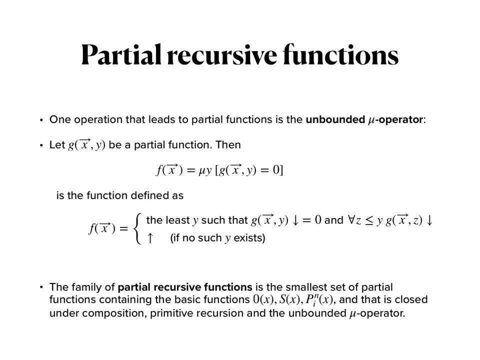 bounded that is smaller than a given bound. Now we get rid of this bound, and this hence corresponds essentially to an unbounded search, which, of course, can lead to an infinite loop if we never find a witness for the condition that we're looking for. So, formally, we have a partial function given. 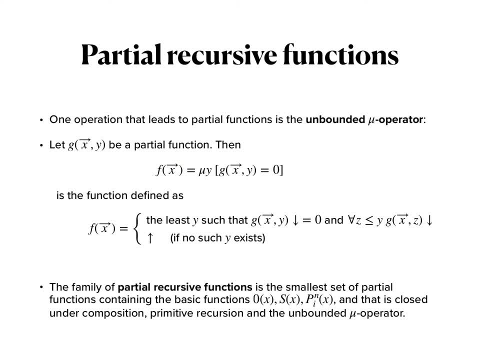 and then the function f, obtained from g by application of the mu operator, is defined as follows: It's the least y, such that g is defined, and zero, And this is important. we also have to require that g is defined for all z less than equal to y. If we don't, 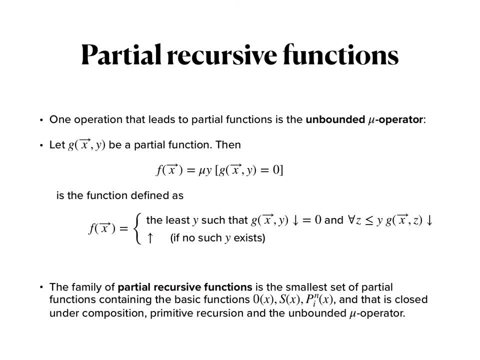 require this, then the partial recursive functions that we define below will not be used under this operator, And if no such y exists, then we just let f be undefined. So and then the family of partial recursive functions is the smallest set of partial functions, containing the basic functions zero, successor and projection, And that is closed. 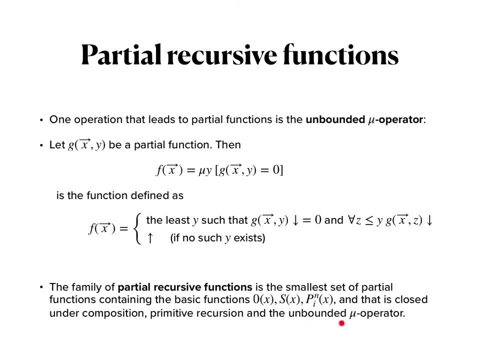 under composition, primitive recursion and now the unbounded mu operator here. And it should be clear how you can adjust the notions of composition and primitive recursion to actually apply to partial functions. So whenever you're, essentially whenever you run at some point of the definition. 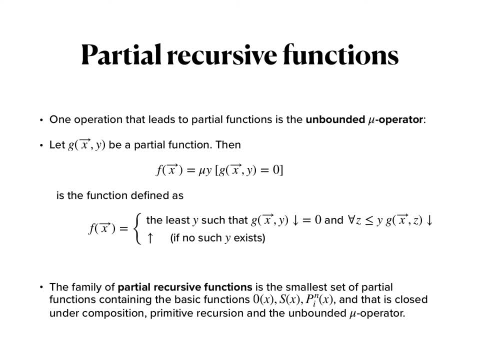 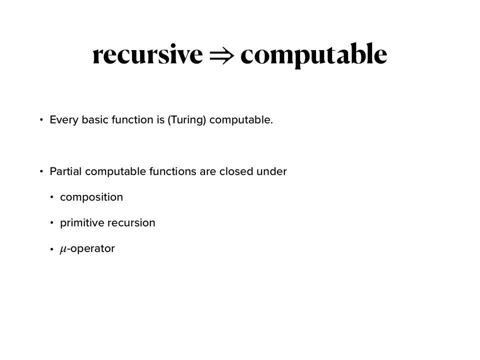 into a partial, so an undefined value. then you just make that function undefined. You carry that undefinedness along in the function that you're currently defining, So that shorter than equal to one- really I mean that's a long termabout. It is now possible to show that every recursive function, or partial recursive function rather, 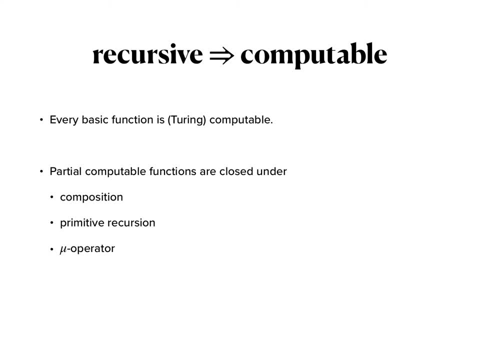 is partial computable, and this works by showing that every basic function is Turing computable. We've already discussed this in class. And then you show that the partial computable functions are closed under composition, primitive recursion and the mu operator, And that means when each recursive is greater that the unbounded mu operator. per villain, This dis donkey work happens in formal þ is. 그런데 this is given by a constant at small. 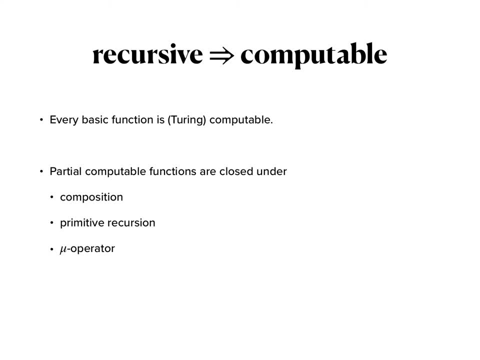 means that the family of Turing-computable, partial Turing-computable functions contains the partial recursive functions, And here you essentially just give a Turing machine that performs these operations, given Turing machines for the functions that you, for example, want to compose, and so on. 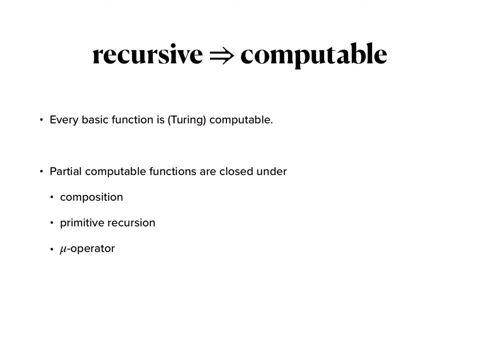 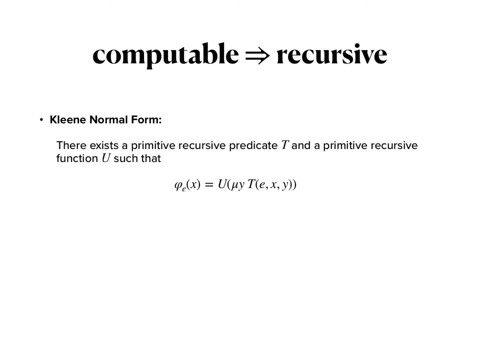 There's nothing really special about Turing machines. here You can do similar, sometimes even easier proof using other frameworks, such as the register machines we looked at, and so on. Finally, you can also show that every partial computable function is partial recursive. 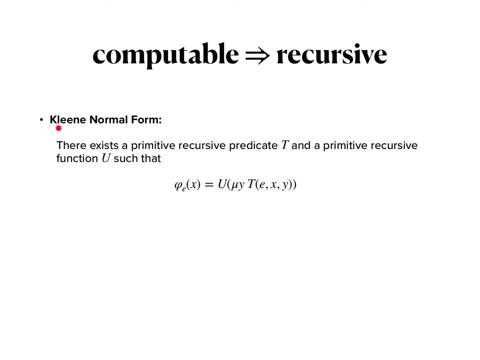 And this can be done through proving what is called the Kleene normal form, which says that there exists a primitive recursive predicate T and a primitive recursive function U, such that the ETH Turing-computable function phi sub E, applied to X. 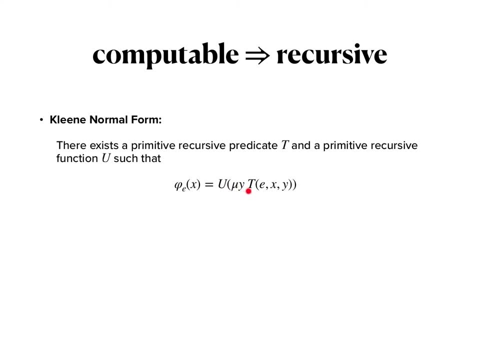 is obtained by applying the mu operator to T and then applying U to the result of that function. So this in particular shows that one application of the mu operator is enough to get all Turing-computable functions from the primitive recursive functions. 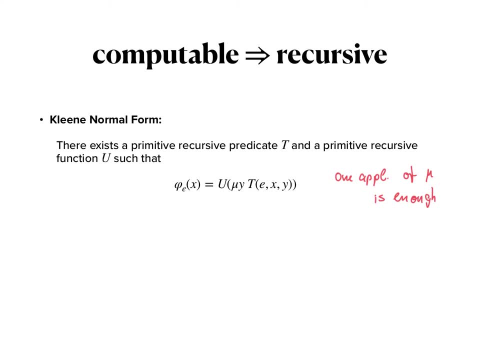 The proof of the normal form takes us back to when we first looked at how we can code Turing machines, And at that time we not only coded Turing machine programs, but we also coded computations of Turing machines. If you recall, we encoded the computation of a Turing machine by encoding its configurations. 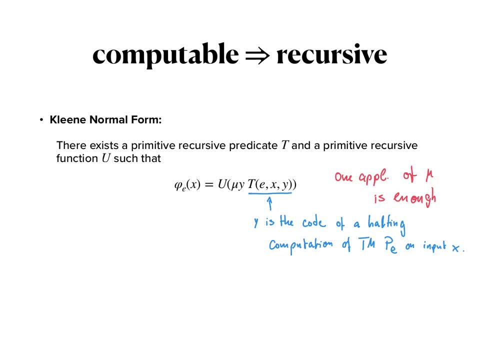 The configuration of the, for example, the position of the read-write head, the symbol that is currently scanned, the state that it is in, and so on, And then that sequence, so each configuration could be encoded by a single number, and then the sequence of those configurations again is a sequence of numbers. 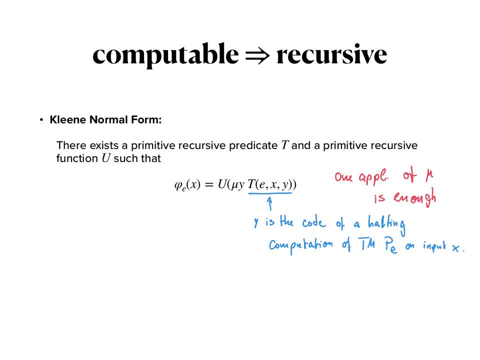 and that could be then turned into a single number. And essentially, this predicate now says that Y is the code of a halting computation of Turing machine phi sub E on input X. Of course, this halting computation might not exist at all. 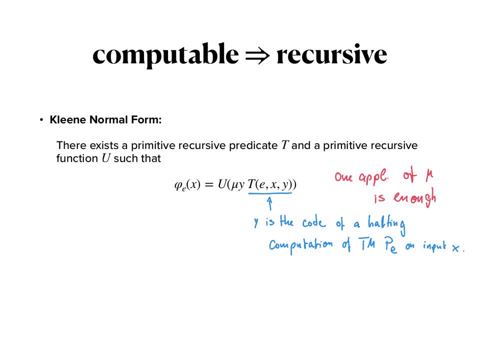 This is why this search, so this mu-operator, might lead to an undefined function, But if it is so, if there exists such a Y, if it is halting, then we can decode the last configuration, namely the halting configuration. 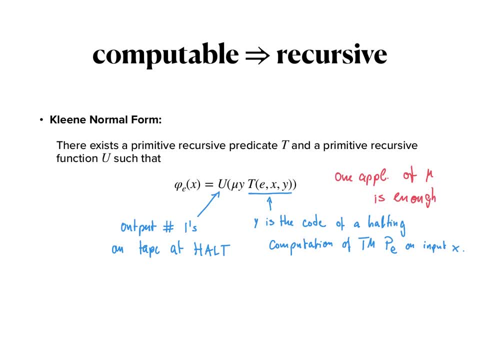 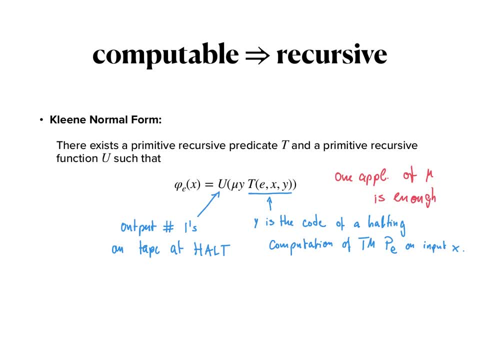 theoretic operations of coding, encoding, decoding and so on are primitive, recursive, and hence they can be used to define these functions: u and t. 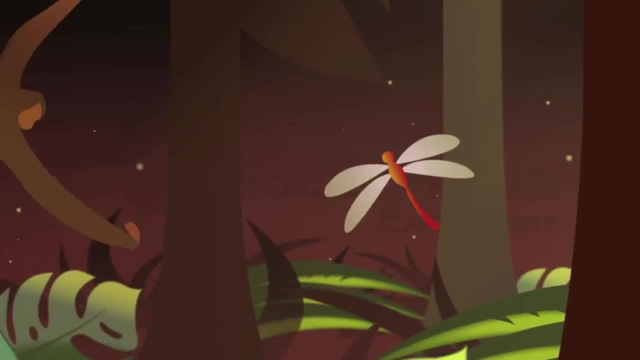 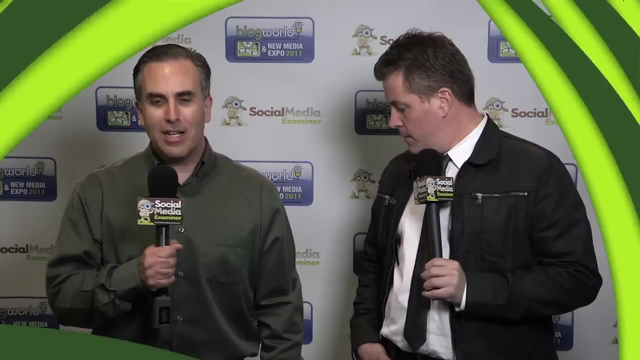 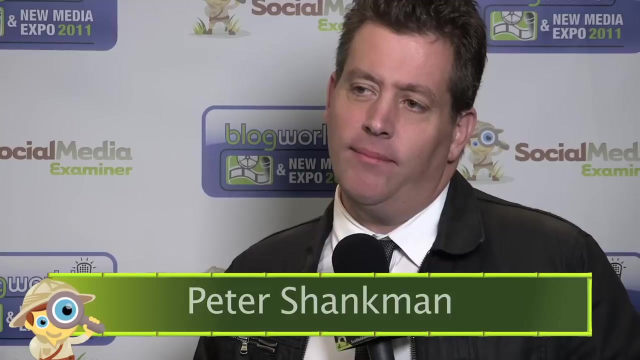 Mike Stelzner from Social Media Examiner, and I'm joined today by Peter Shankman, who's the founder of Help, A Reporter Out, also known as HARO, and he's also a vice president at VOCUS. Correct, How are you doing today? 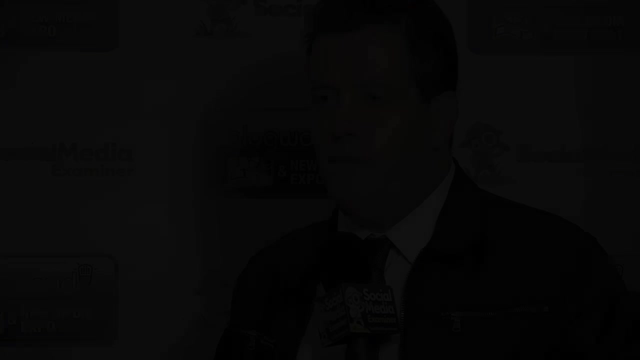 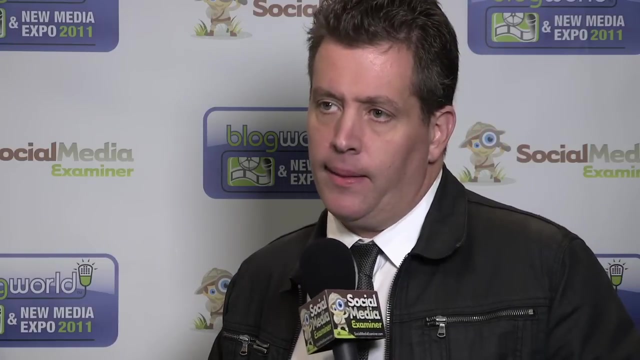 I'm doing well myself. Excellent, thank you. So let's talk about HARO. You can argue that HARO was an early social network because you were connecting experts with the media. How have things changed in social networking since you started? 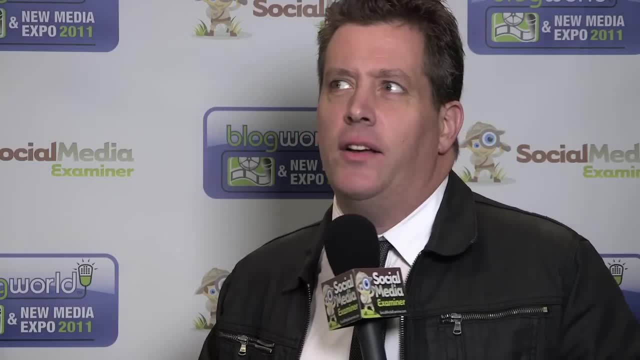 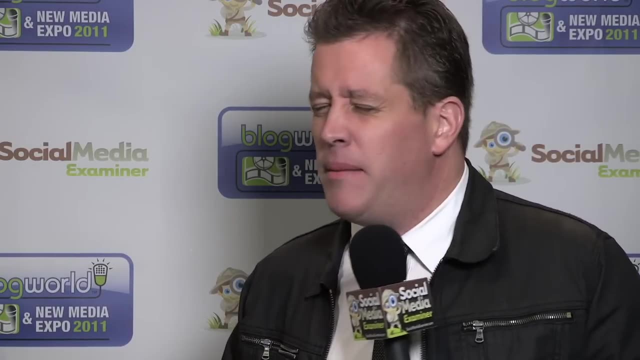 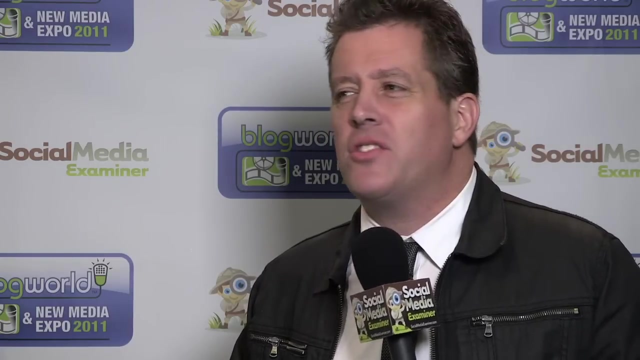 There's no doubt we were a social network right at the beginning. We were one of the first social networks that really connected journalists with sources, and did so in such a way that it just exploded to over 200,000 people now What it becomes is what we're seeing now is so many different social networks and so many ways of information flowing in. you have to continue to be relevant to your audience, because it's so easy to get distracted now and go somewhere else. there's no loyalty anymore. 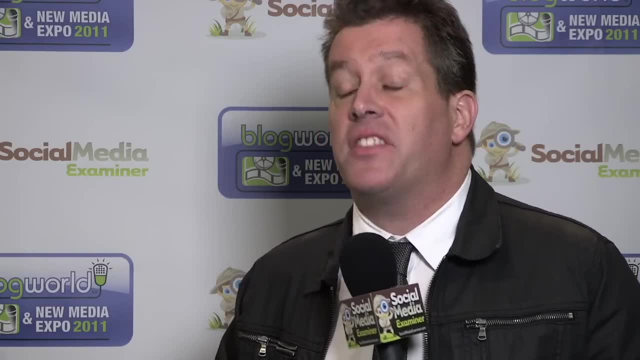 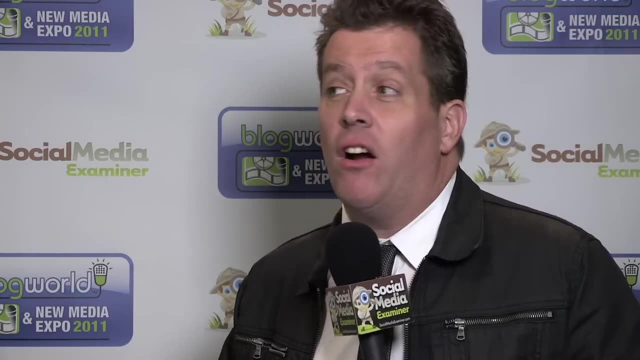 You have to. You have to be relevant to your audience. HARO comes out at the same time every day with the exact same types of queries. you know we don't change, we evolve, but the consistency is there and our users, our customers, love that from us. 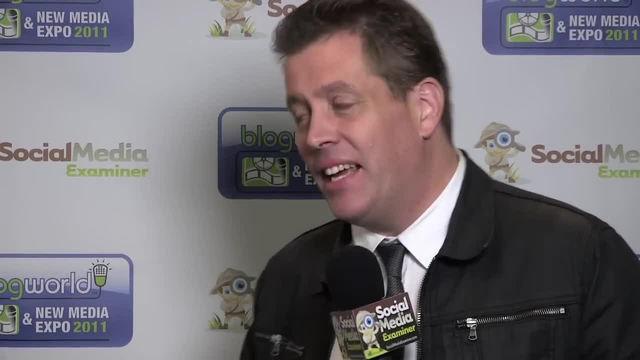 Interesting And I'm just like, well, you know, okay, I guess I was on to something Exactly, And we really blew it up and it really had a blast with it. Yeah, Yeah, Yeah, Yeah Yeah. 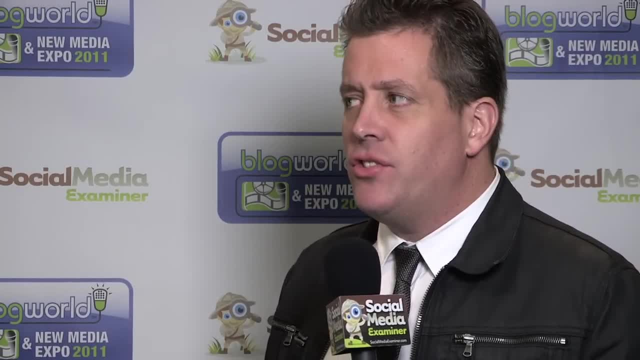 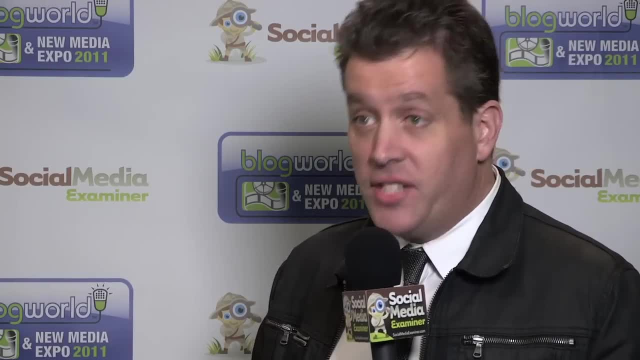